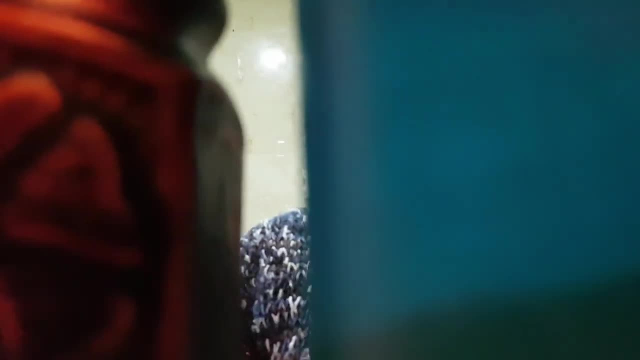 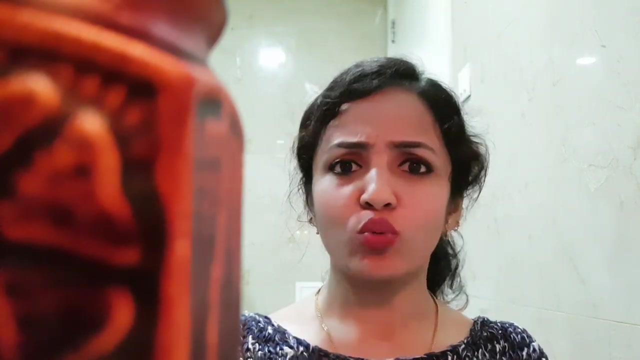 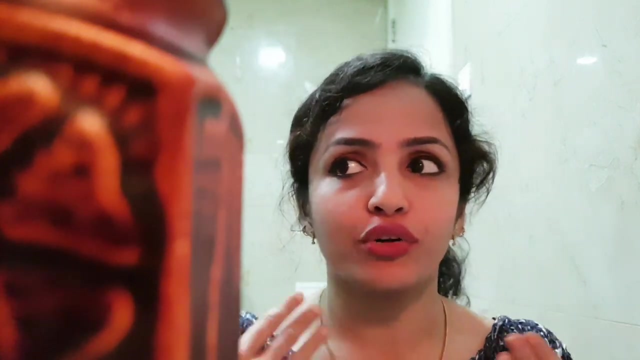 Hello friends, welcome to your channel. Simply Home Refrigerator is like one of those dumping yards in your home. right, We keep loading stuff inside our fridge, let it be leftover food or fruits, vegetables, etc, etc. Well, today I'll be talking about refrigerator. 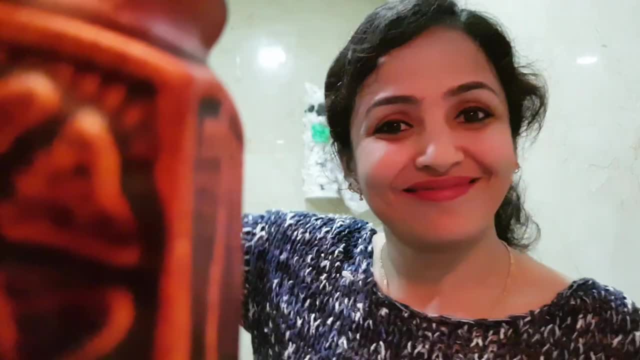 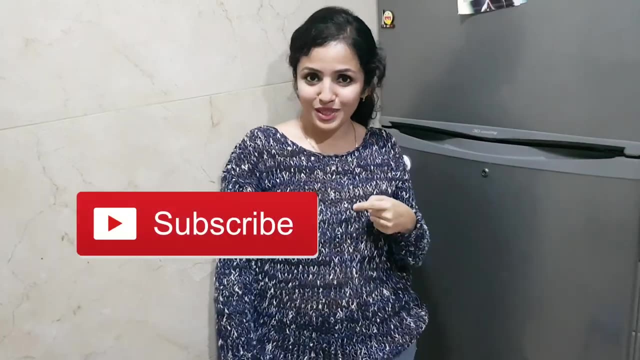 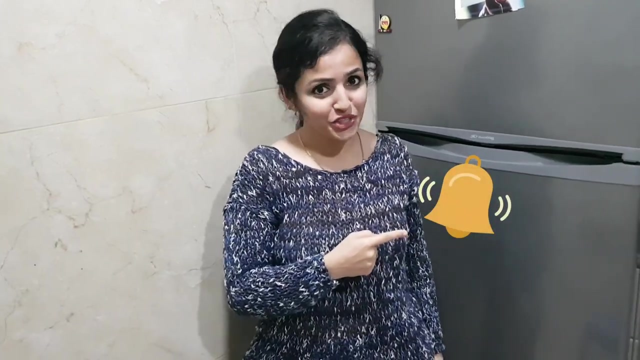 organization, but with a perspective. Just a quick reminder: if you have not done so already, subscribe to Simply Home for more organization and lifestyle videos. Also, click that bell icon to get notified whenever we upload a new video. I'm sure you guys have. 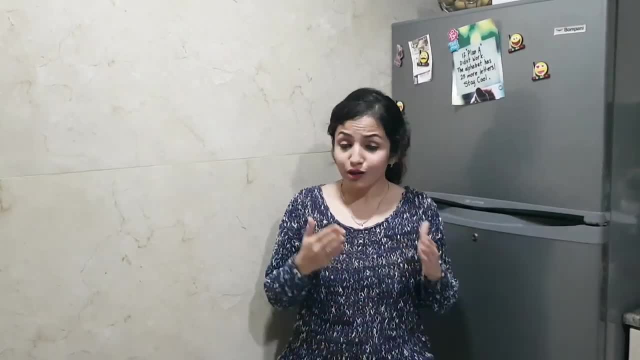 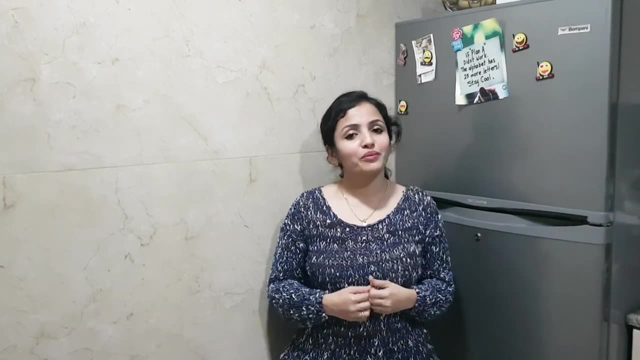 seen many videos on refrigerator organization, how to categorize your stuff inside the fridge, etc. etc. Well, this is a pre-loved fridge. We bought it from a very dear friend of ours when we first moved into the UK. The brand 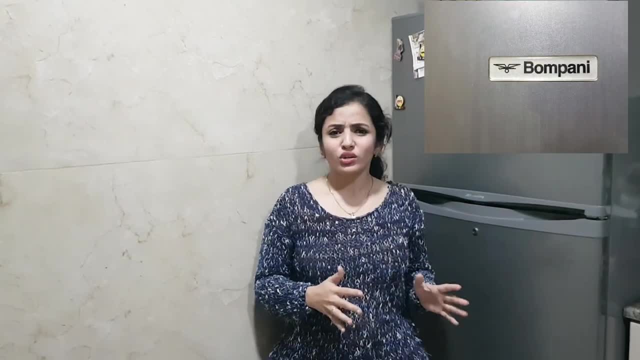 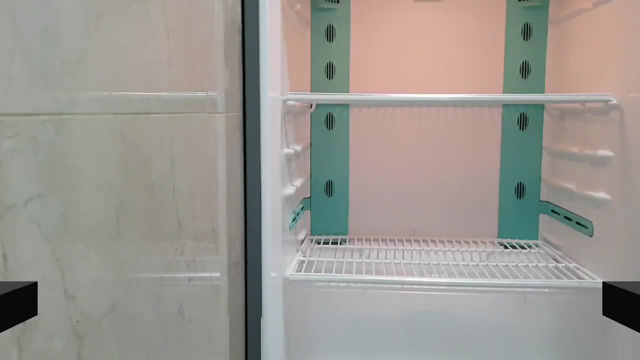 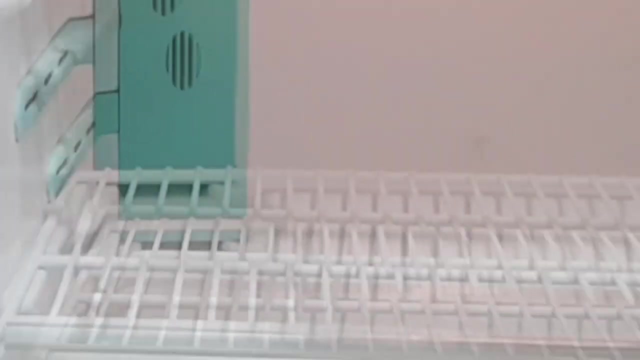 is Bompani and it's a double-door fridge. I'm not sure what exactly is the capacity in numbers and units, but I can say that it is a very spacious one. As you can see, our refrigerator had only two racks. The vegetable box cover was missing, So I placed the second. 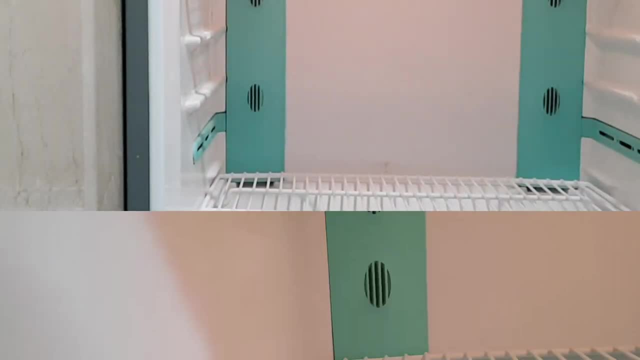 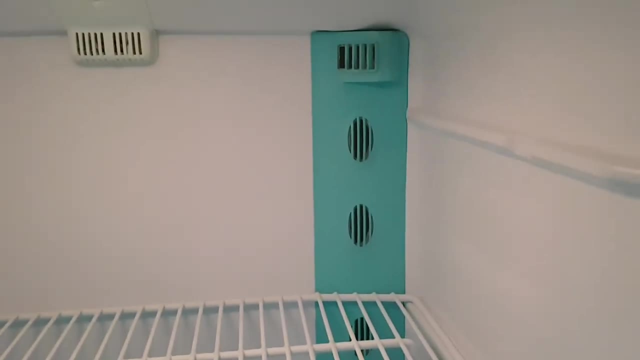 rack on top of the vegetable box only to give it a finished look. The advantage of a refrigerator was it was comfortable. The refrigerator is a lot more spacious and deep than a fridge. I just didn't have enough racks to use that space. We haven't thought of replacing her yet, because she has stood. 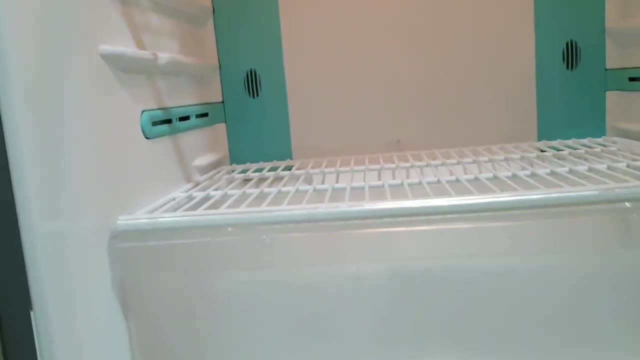 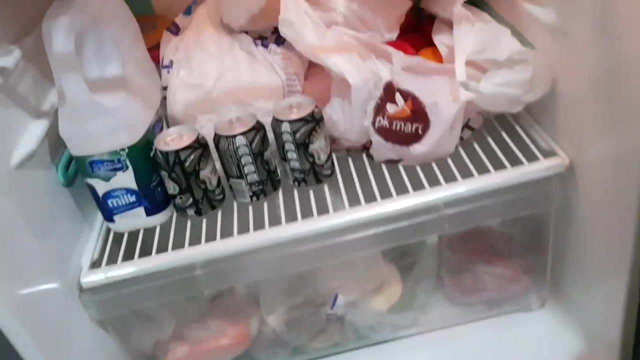 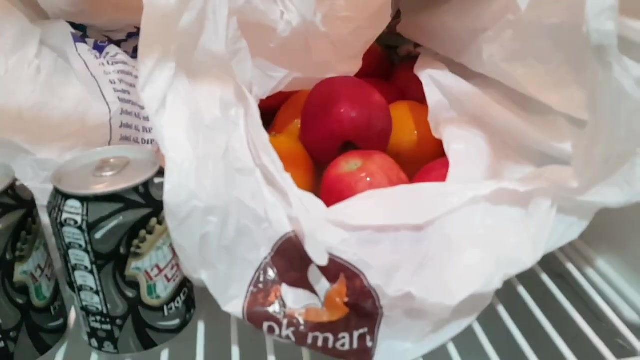 by us quite faithfully for the past five years, except for a few hiccups, But nothing big. We usually buy fruits and vegetables and other consumables for a week at once. Out of this, fruits and vegetables need to be refrigerated to keep them fresh for longer. I also bring. foodstuff back from my hometown in bulk for the next few months. We have lots of things to do and we need to go out and have a good time. I'm looking forward to getting ready for a day or two, But I will be back with a video soon. Let's get started. Let's get started. 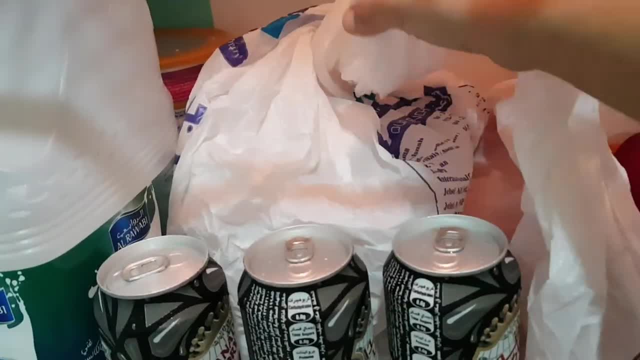 1. Refrigerator and refrigerator. 2. Refrigerator refrigerator. 3. Refrigerator refrigerator. 4. Refrigerator refrigerator bulk, which also needs to be refrigerated for longer life. I had a vegetable box to store my veggies. 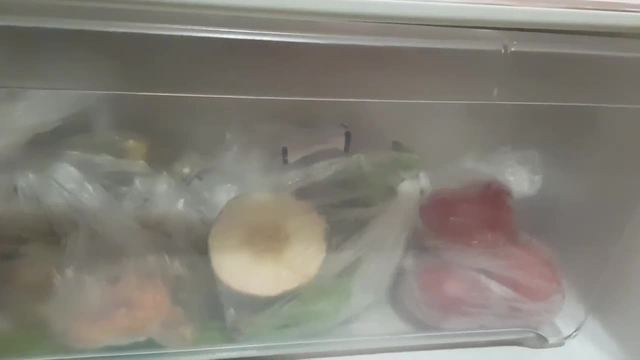 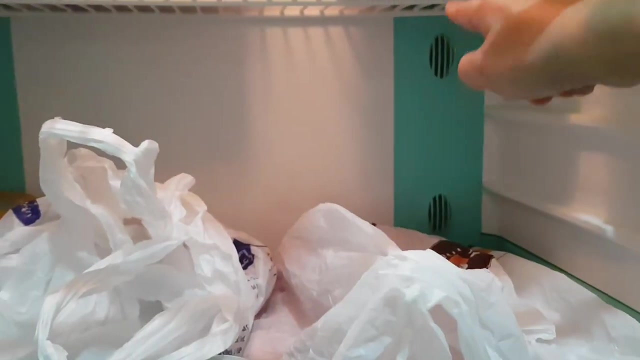 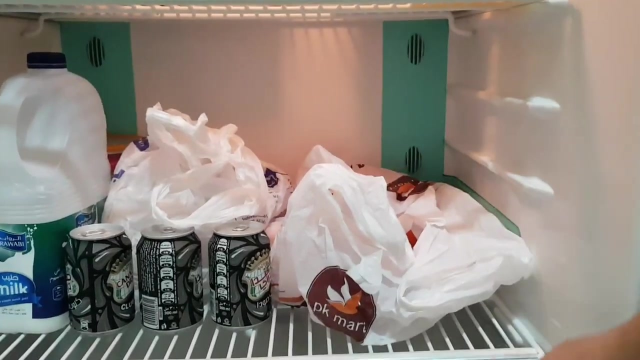 I needed a system for my fruits. I tried using polythene covers to keep them segregated. It worked okay, except all the space between the fruits and the upper rack remained unused and the whole place looked messy. I couldn't put it in my vegetable box as well, as it will be overstuffed. 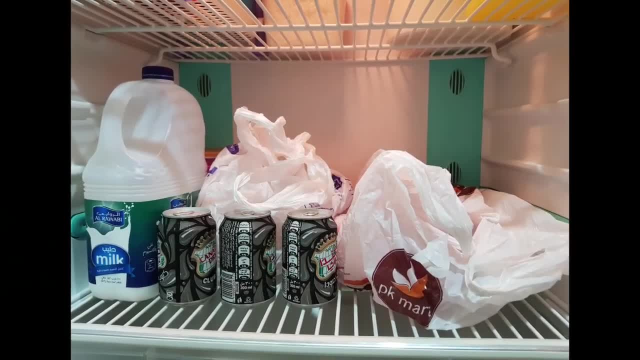 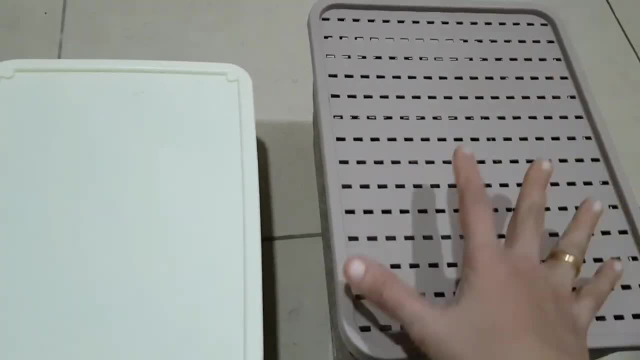 I needed a system that would help me keep everything organized and put together. This was the solution that I found. I bought these two baskets from Amazon India. I have provided the link in the description box down below. I got it at a pretty good deal. 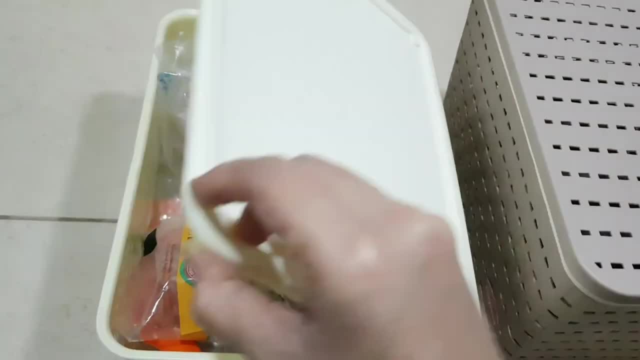 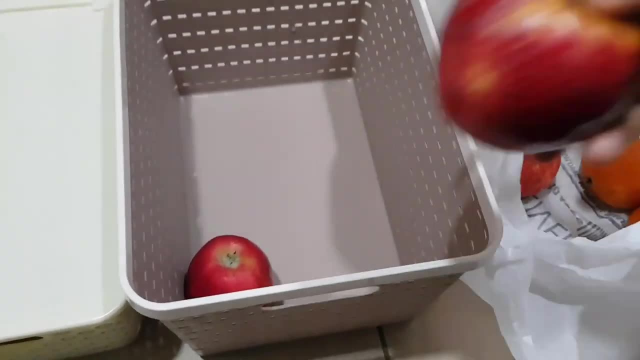 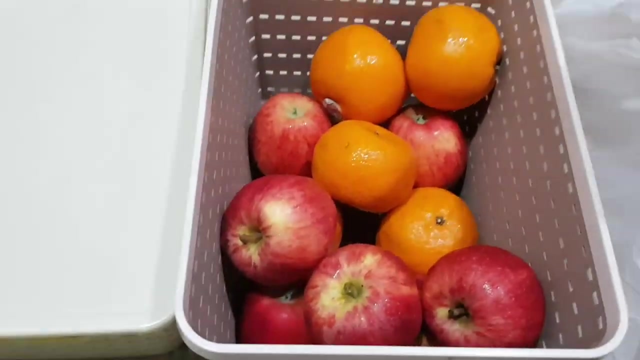 Since these had lids on it, I could easily stack them one above the other and use the vertical space in my fridge. I used one basket to store the foodstuff I bought from my hometown and the other one to store fruits. Both the baskets were well ventilated, allowing ample airflow inside and out, allowing the 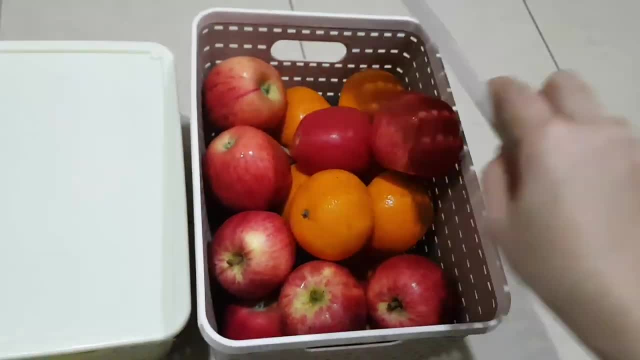 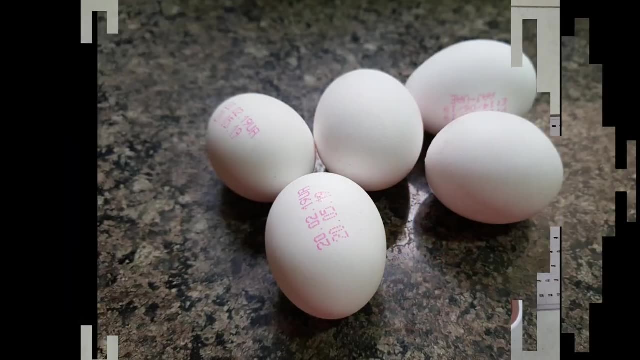 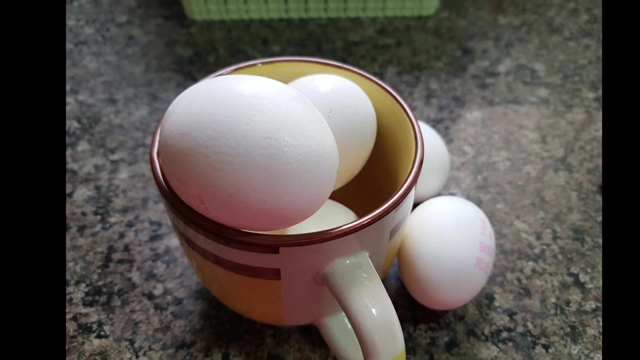 foodstuff inside to stay fresh for a longer period of time and my problem was solved. Eggs are one of the other things we buy in bulk. Being fragile makes it quite difficult to store. My refrigerator egg tray had option to store only 8 eggs, so I started storing them in the 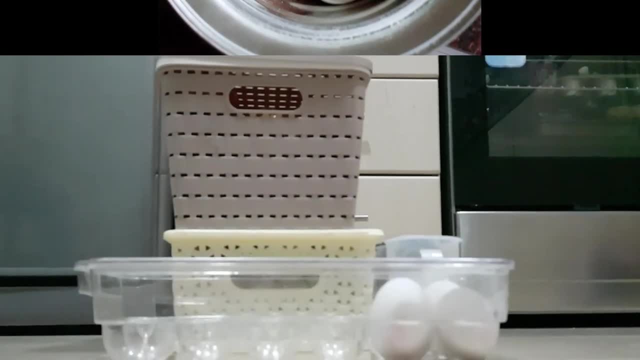 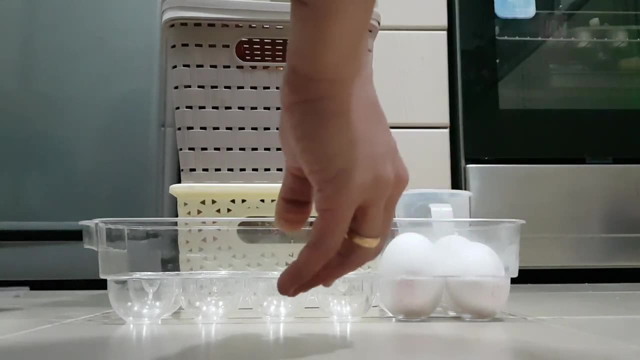 used formula tin of my baby. It's a pretty good DIY, by the way, if you want to try it out. The problem was the eggs started getting cracked when I had to move the tin- to take out the eggs or just to move it out of the way. 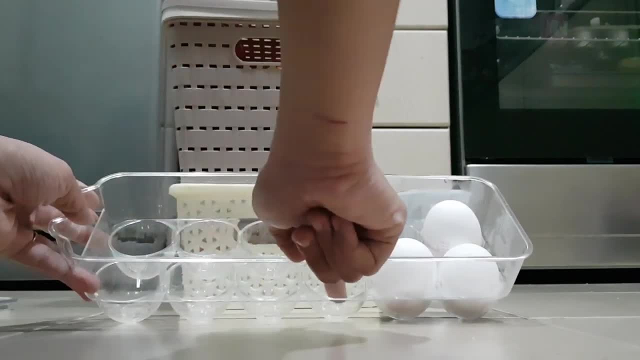 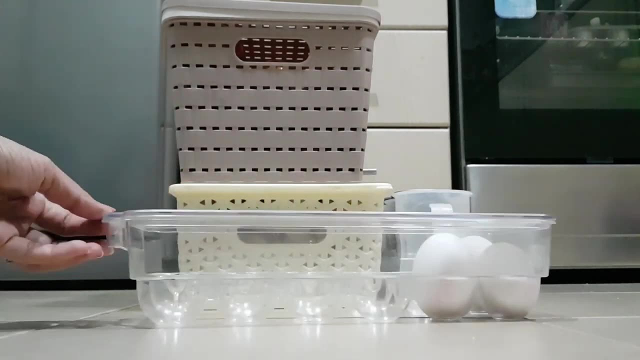 So I bought two of this egg tray from Homebox UAE. It has an option to store 12 eggs in total. It's quite sturdy, stackable and sleek. It will slide right in my fridge and it's quite easy to pull out with that pull out. 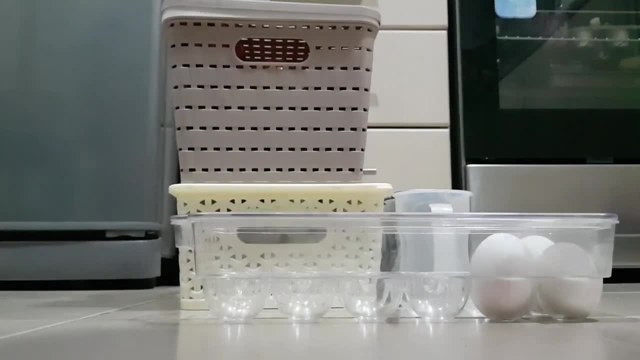 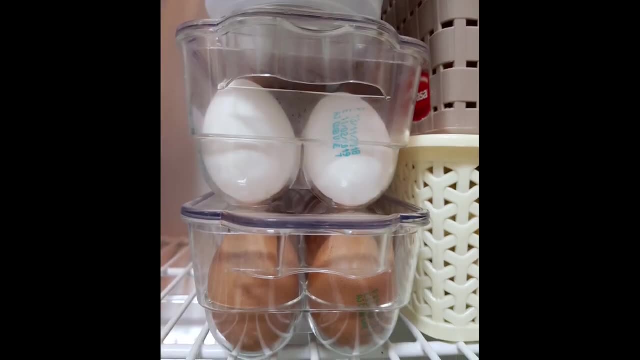 knob. Since I bought two of these, I could easily store 24 eggs at a time. I have put all the links of the organizers that I bought online in the description box below, in case you are interested to check them out. For those of you guys who like storing and taking out coke and soda cans with you, this: 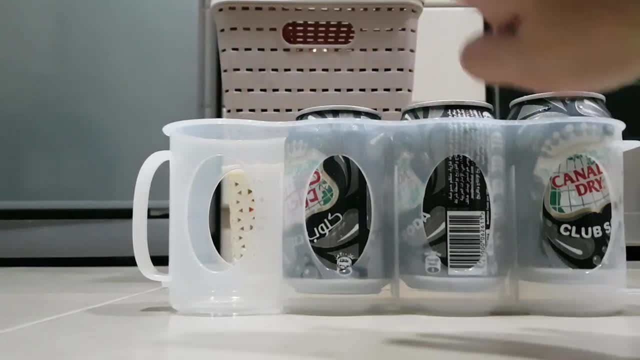 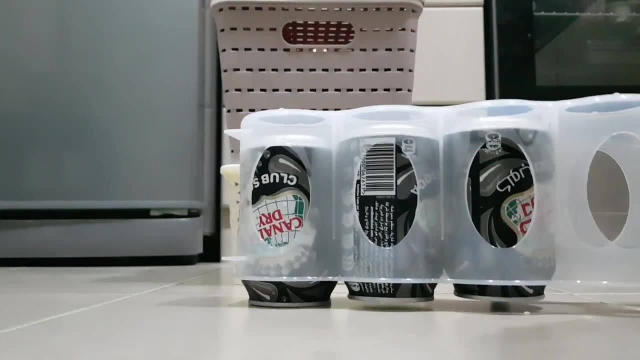 can organizer will get you sorted. It has an option to store 4 cans at a time. It's quite easy to slide in and out of your fridge. It has a handle at the end which you can use to carry out when you are going for picnic. 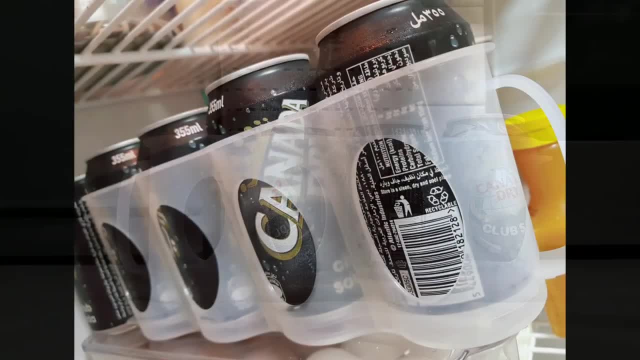 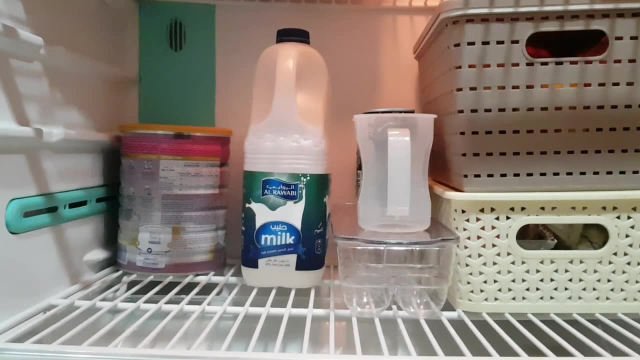 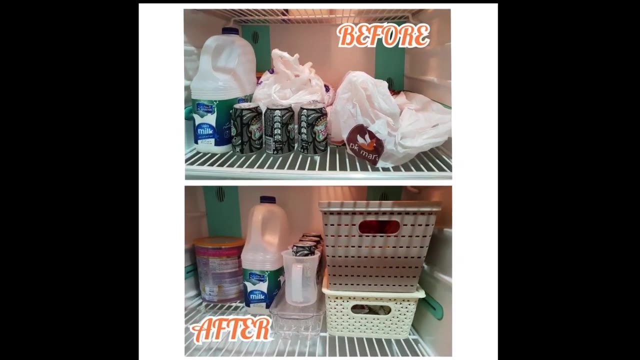 or an outing Guys. this is the final look of the lower rack of my refrigerator. I could tackle all my organization issues quite successfully. As you can see, the clays looks quite put together and mess-free now. Now coming to the next part: storing leftover food. 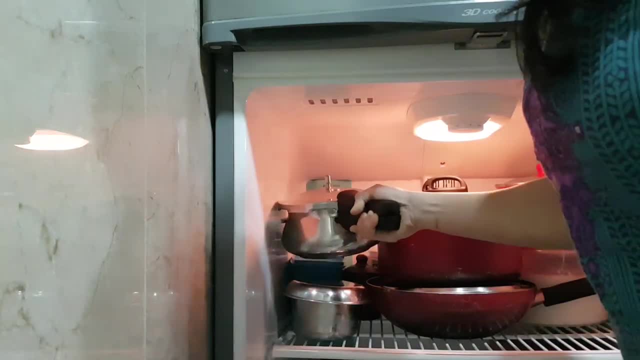 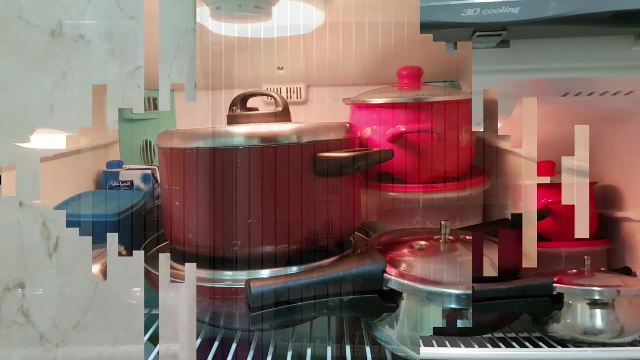 I used to store my leftovers in the pots and pans. I cooked them in, thinking it was easier for me to reheat them the next day. This method worked fine for us for some time, but soon we started facing space constraints. I started storing leftovers in smaller containers. 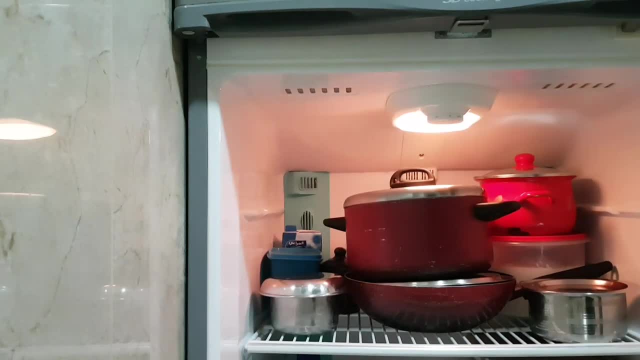 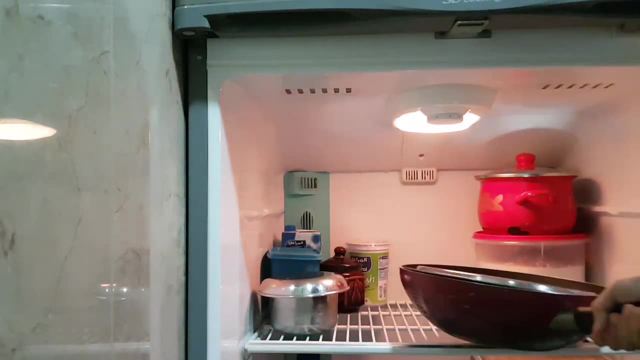 Again I faced challenges, since my fridge had only two racks and all the vertical space was lost. I couldn't stack the containers one above the other, as they would lose balance and spill out the contents. In the end, I tried Tupperware containers, which solved my problems. 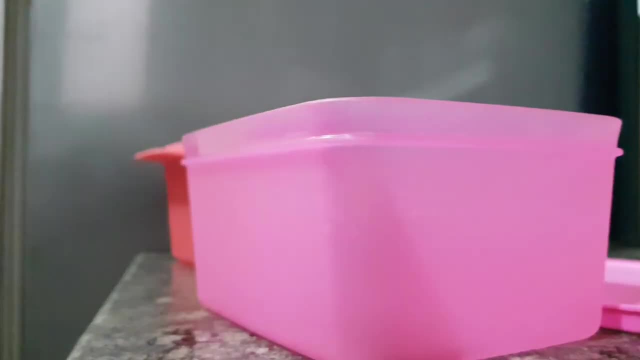 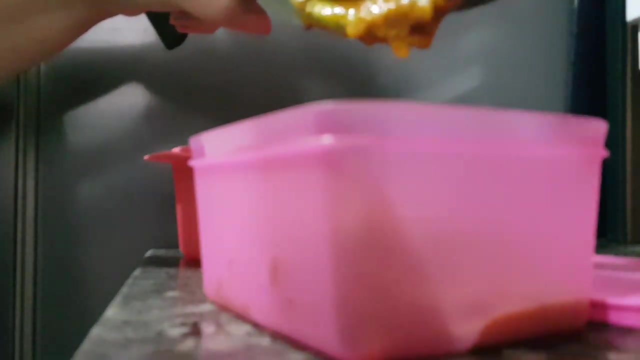 These are stackable, airtight and liquidtight containers made of plastic. These containers are made of plastic. These containers are made of plastic. These containers are made of high quality food grade plastic. My advice to you would be to always go for containers like this, which are not fancy, since 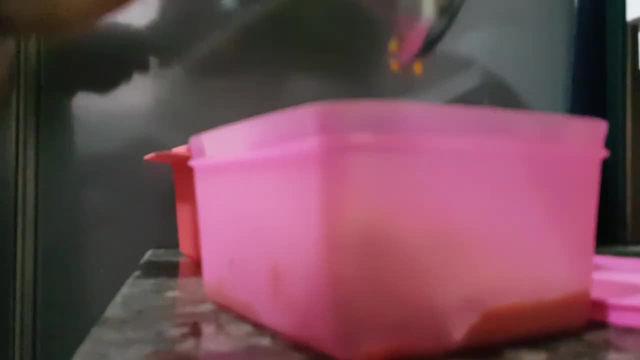 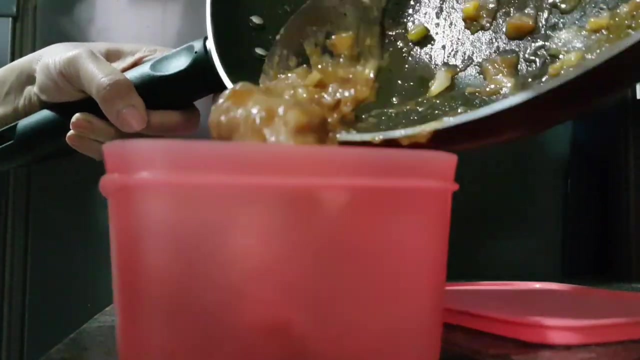 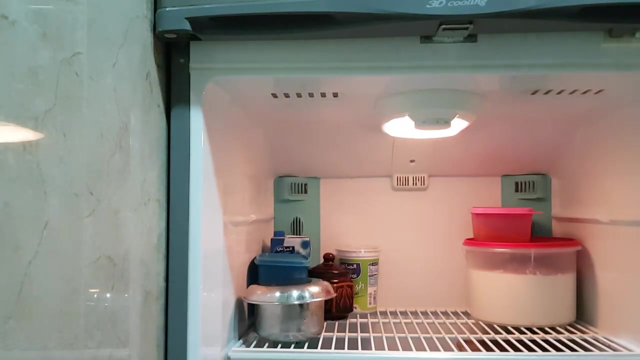 fancy containers take a lot of dead space. A small health tip regarding plastic containers: however high quality they are, store your leftovers only after they have completely cooled down. It definitely looks as if my fridge has got some air to breathe now. As you can see, these containers are stackable and sleek, saving a lot of space inside my 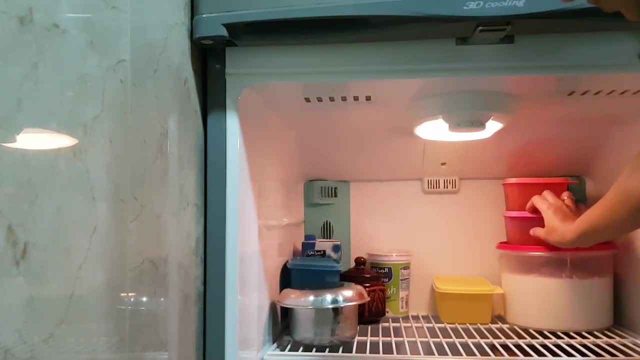 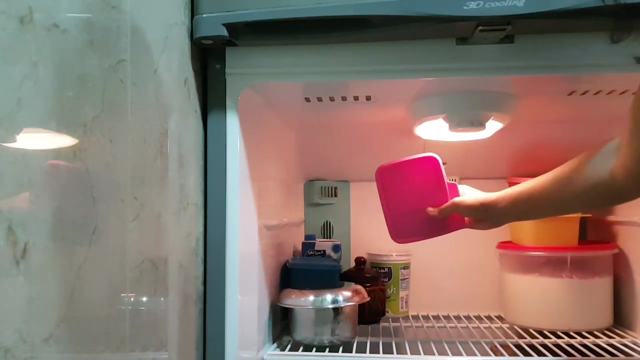 fridge. You can stack them up anywhere, one above the other. The primary reasons why I went for Tupperware containers is definitely its quality, But apart from that, since it's airtight, the risk of cross-contamination is minimal, and since it's watertight, the contents will not get spilled out if it falls down by accident. 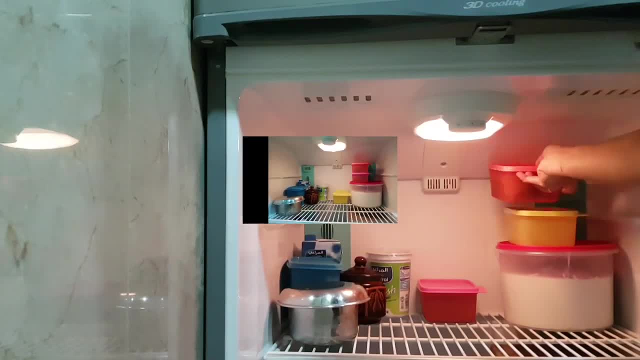 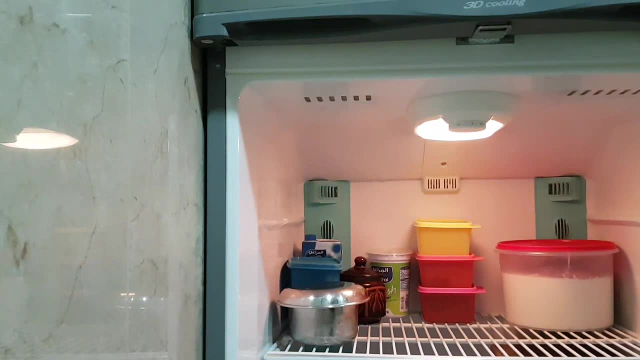 So, guys, doesn't this place look quite put together? Let me know in the comments below. Thanks for watching. It's been a while since I've done a video on how to store containers. These containers look quite put together now. Still, I felt there was still scope for vertical space utilization in this area. 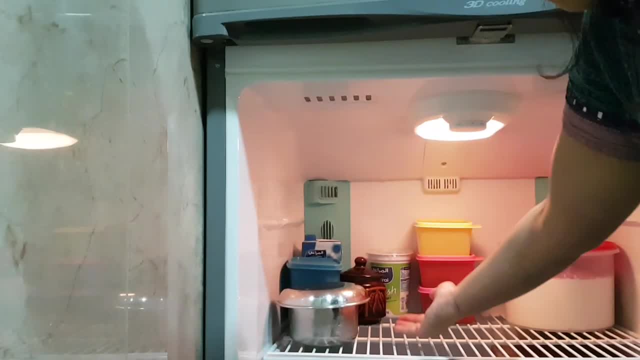 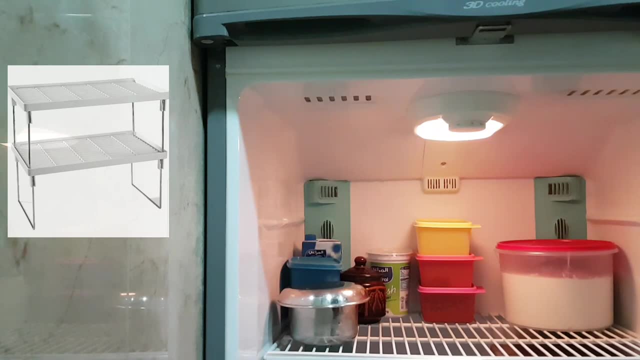 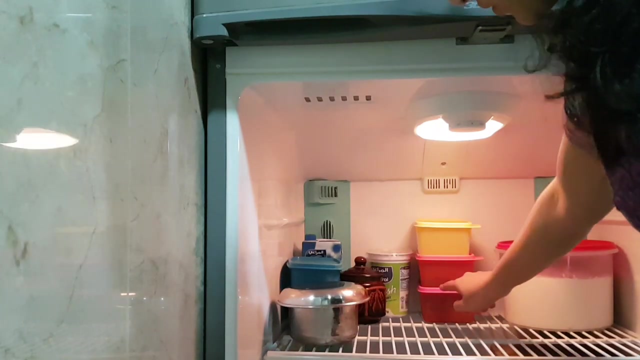 As I mentioned before, my refrigerator had only two racks and I was dying for more storage. I couldn't use my folding rack for obvious reasons. I didn't want to risk my corner rack getting rusted as well. If you guys are wondering what the corner rack and folding rack are, please do check my video. 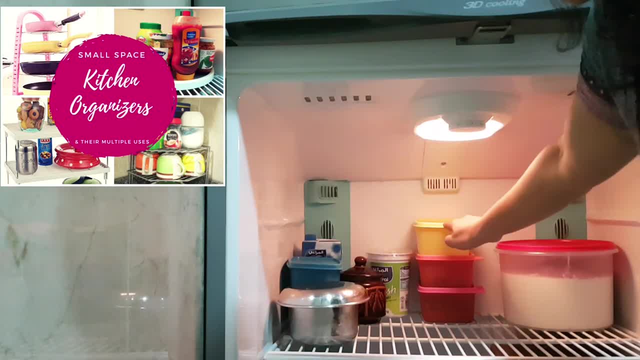 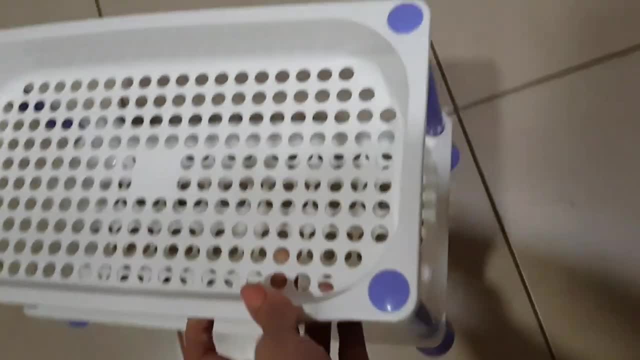 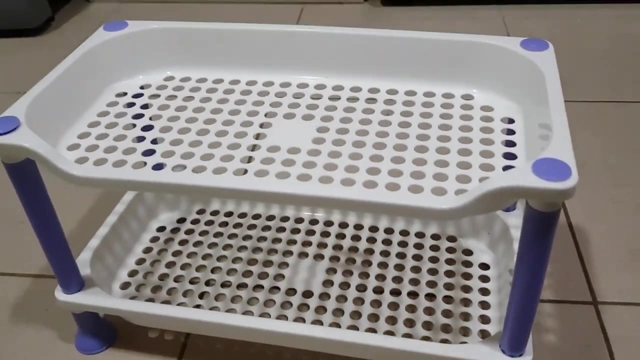 on useful kitchen organization. I've put the link down in the description box below. So I came up with this. It was an idea in the beginning, but it worked perfectly fine for me. It is a three-tiered stand which I brought from a Tendurum shop. 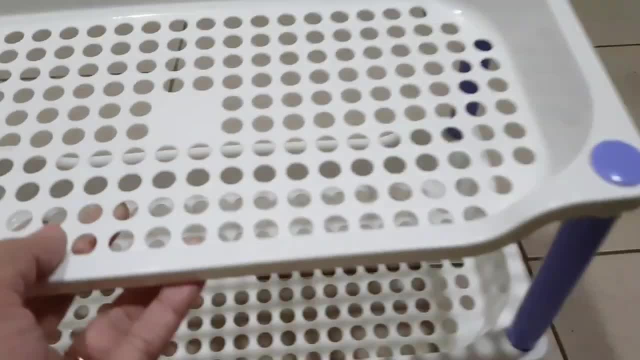 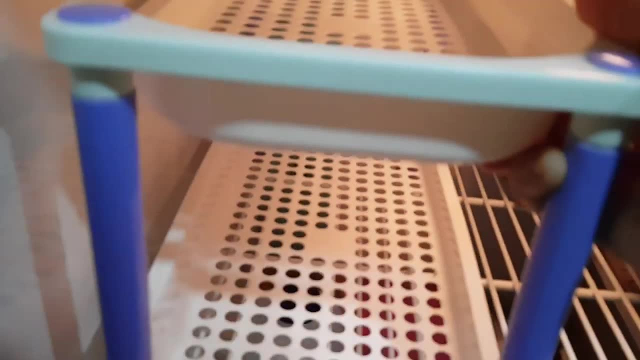 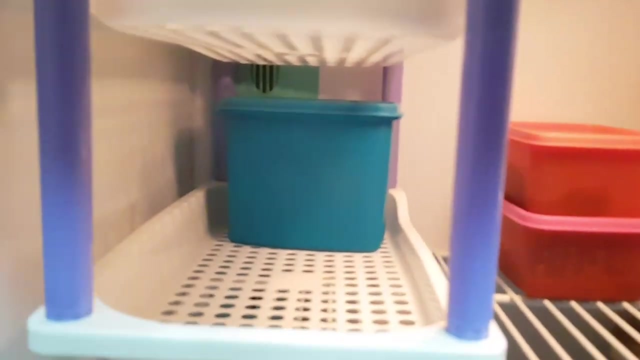 A Tendurum shop is a discount shop in UAE. It is much similar to a dollar store in some other part of the world. Only two tiers of the stand was enough in my refrigerator to keep my things organized and segregated. As you can see, my tins fit perfectly inside the stand. 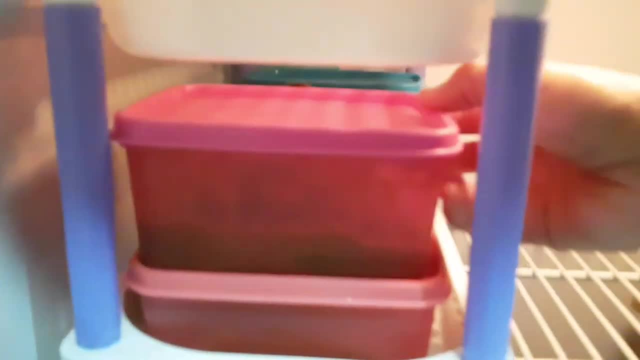 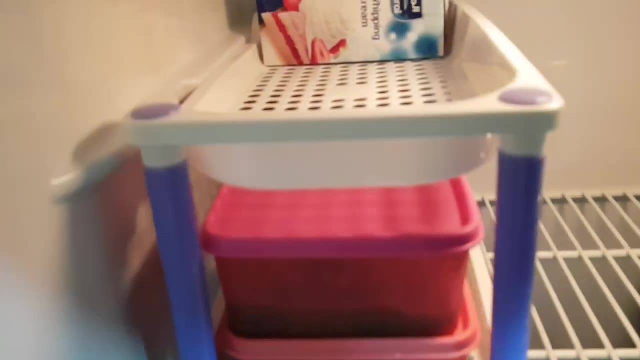 I am able to use that vertical space. I am able to divide that vertical space and create more storage in my refrigerator. Each and every one of the organizers in my refrigerator is a result of careful assessment and analysis of the challenges that I had to face. 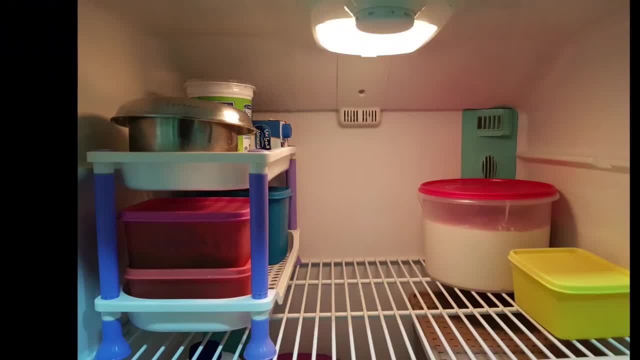 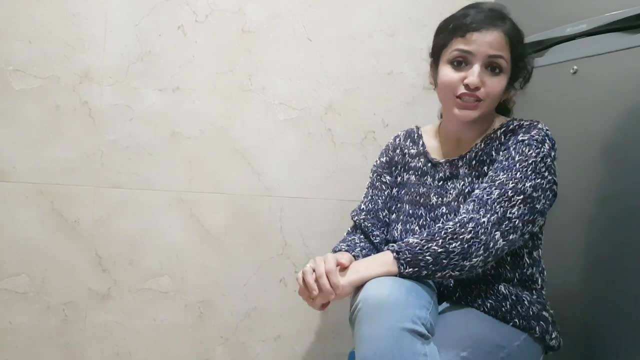 I really hope that this video was able to give you at least a few useful tips on how to maximize your refrigerator space. I'll see you in the next video. This was how I solved my refrigerator organization challenges. So did you guys face any similar issues? 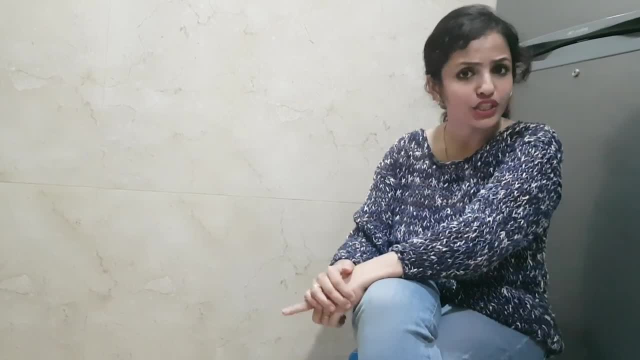 If you did, how did you solve them? Let me know in the comment section down below. We would love to hear from you. Also, if you have any kind of organization problems which you would like to get sorted, please don't hesitate to connect with me on my Instagram or my Facebook, or just simply. 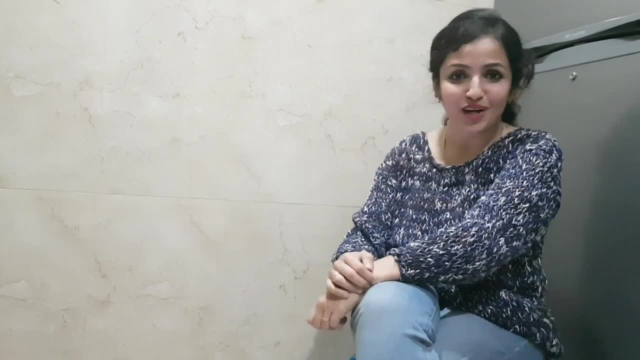 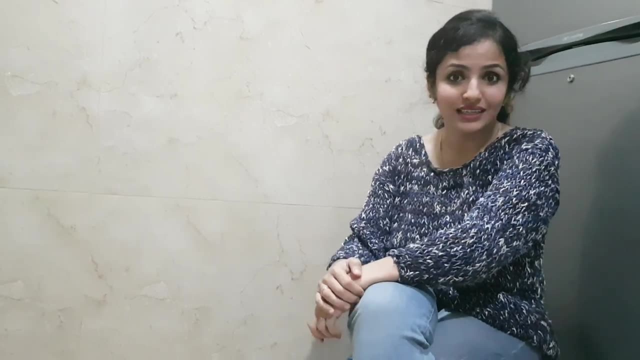 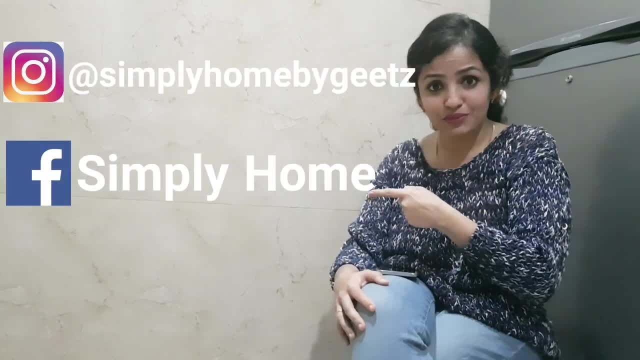 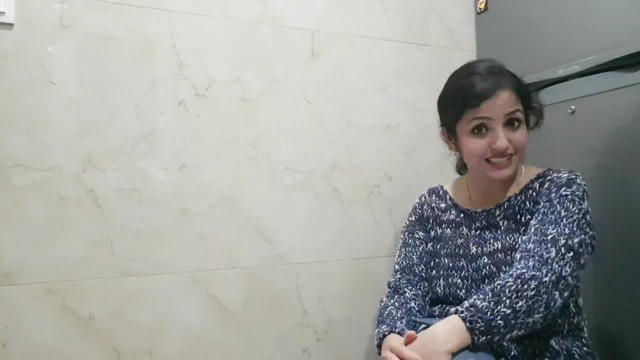 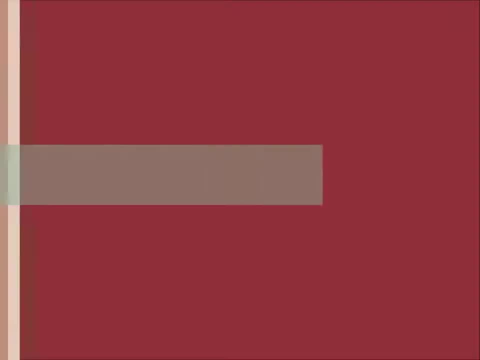 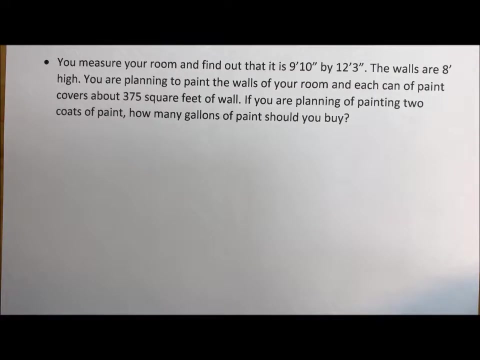 Hi, welcome to Wear Math. Today I'm doing a series of videos on estimation. Okay, you measure your room and find out that it's 9 feet 10 inches by 12 feet 3 inches. The walls are 8 feet high. You are planning to paint the walls in your room and you know that each